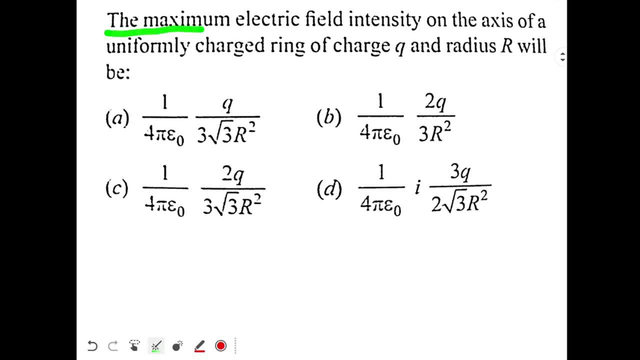 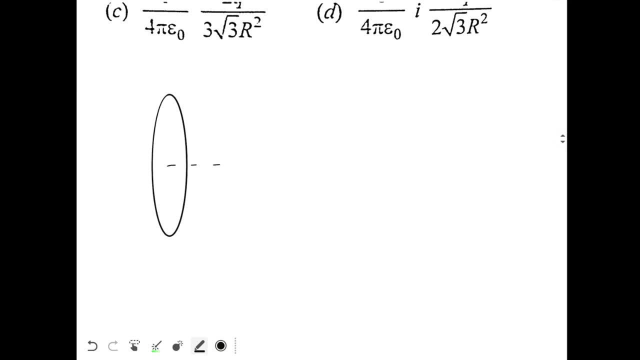 Okay, in this question we are asking the maximum electric field intensity on the axis of a uniformly charged ring. of charge Q and radius R will be what Four options are given. So first of all, we look at the field due to a ring on its axis. So this is a ring and 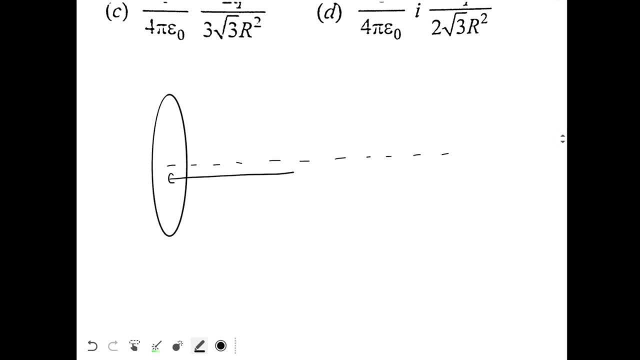 this is the axis of the ring. Okay, the distance X is given by X along the ring. Okay, so the ring will create electric field in this direction, E, and this E will be given by Q, X divided by four. pi. epsilon naught R square plus X square power, three by two, where R is the radius. 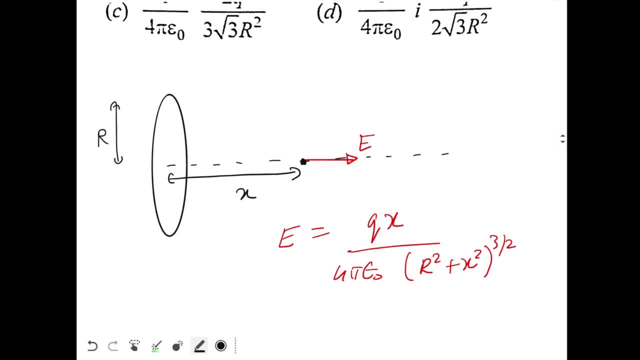 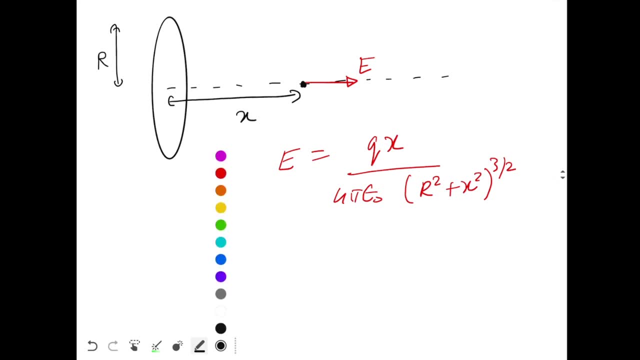 of the ring. R is the radius of the ring. So to find maximum value of E, we need to find a maximum minimum concept, that is, DE by DX should be zero. E is a function of X, so the point where the DE by DX will be zero will give you maximum electric field. So that's. 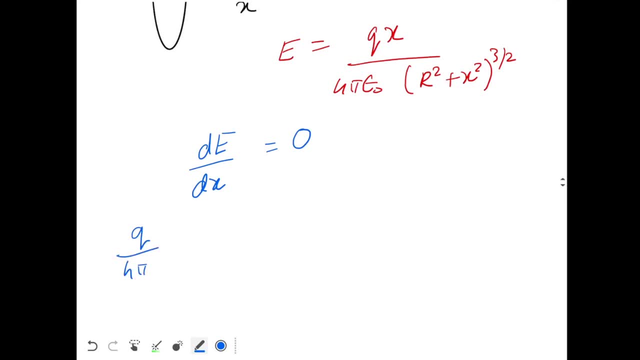 simple. So Q by four pi epsilon naught is a constant. we keep it outside DE by DX of X R square plus X square power minus three by two. This should be zero. Okay, so this part is not required. We take it on the other side and it is gone with the zero. So we just differentiate this. 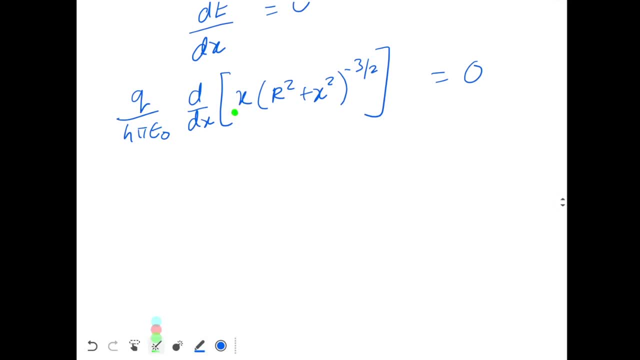 we apply product rule, So first we differentiate x. So derivative of x will be one R square plus x square power, minus three by two plus x times. Now we differentiate this term, So first we differentiate this power. So minus three by two R square plus x square power. 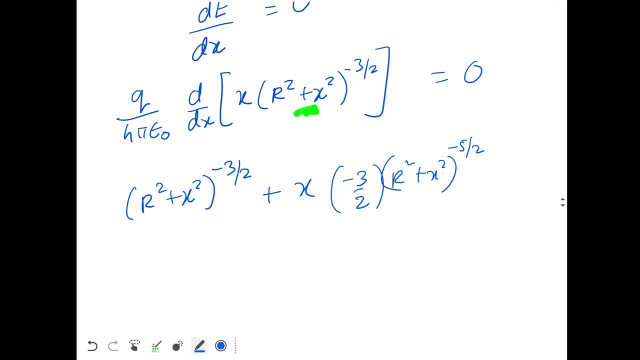 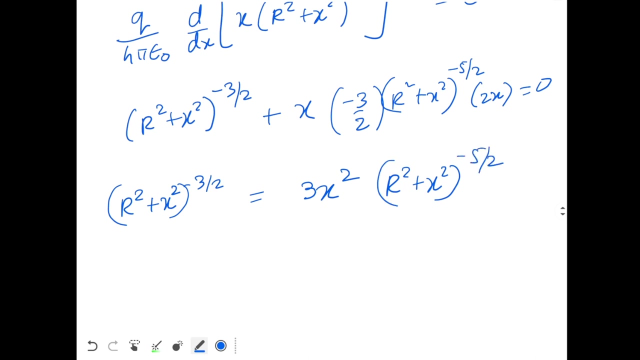 then minus five by two, And finally we go inside the bracket and we get two x. this is equal to zero. Okay, So you will get R square plus x. square power minus three by two is equal to three x square R square plus x. square power minus five by two. Or when you take